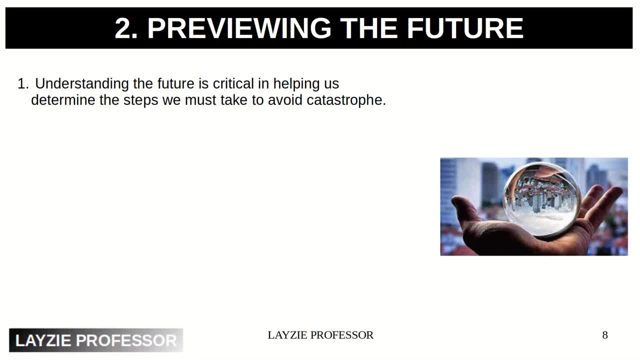 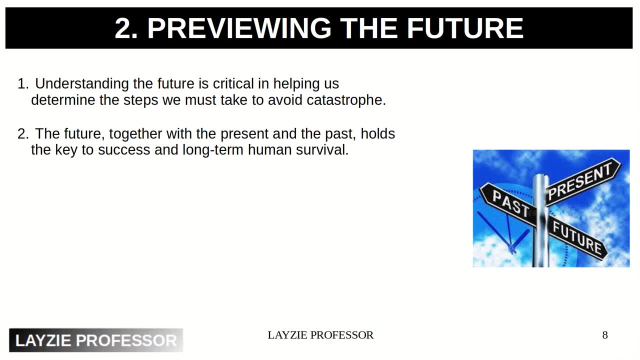 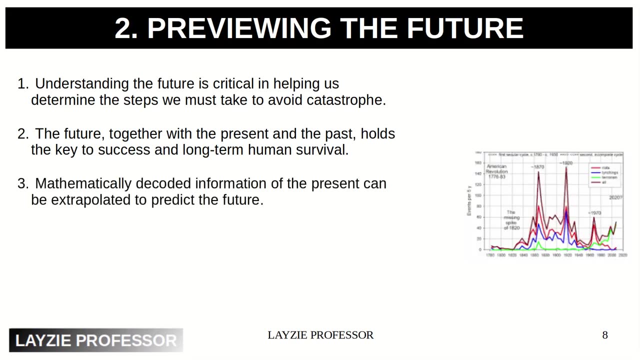 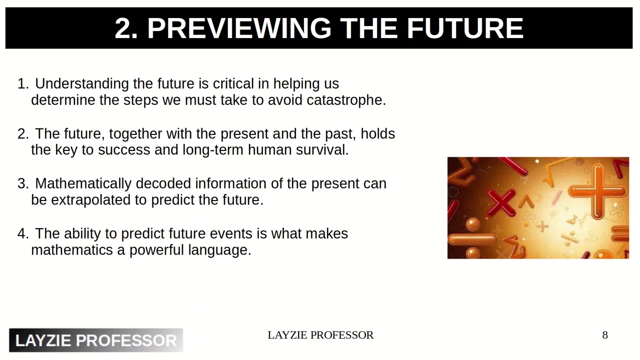 determine the steps we must take in order to avoid catastrophe. The future, together with the present and the past, actually holds the key to success and long-term human survival. Mathematically decoded information of the present can actually be extrapolated to predict the future or future events, and the ability to predict the future is one of the main things which makes 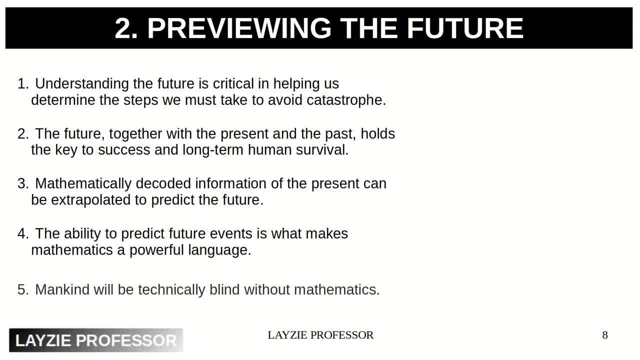 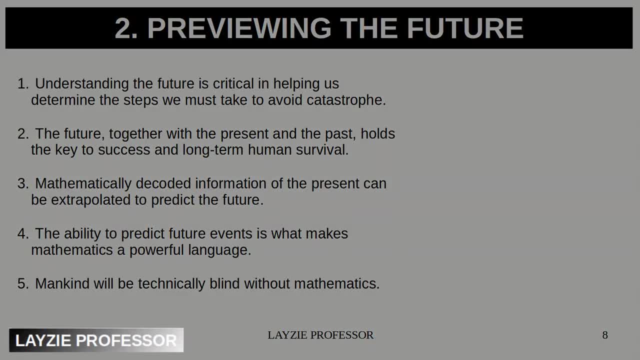 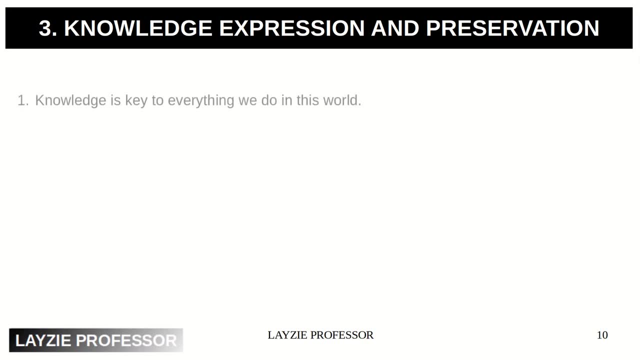 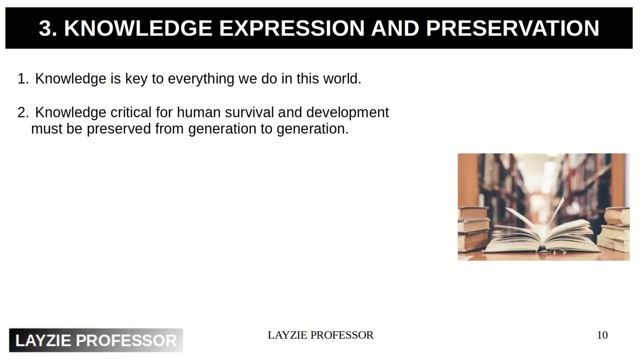 mathematics such a very powerful language. Mankind would be technically blind without such a language like mathematics. Knowledge is key to everything we do in this world. Knowledge, critical for human survival and development, must be preserved from generation to generation. Mathematics is a great tool for 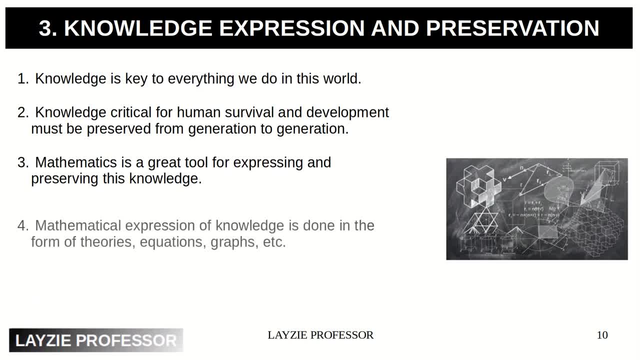 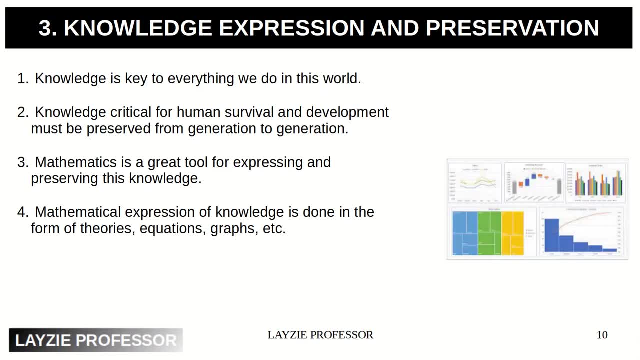 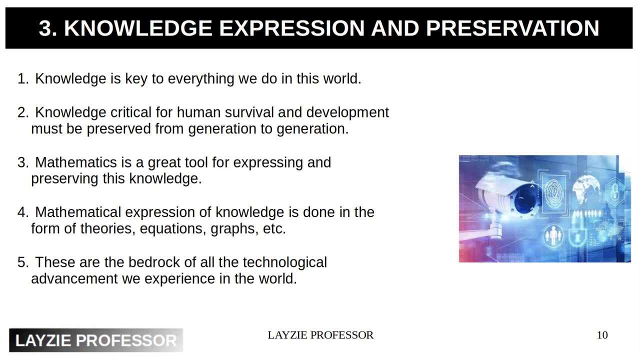 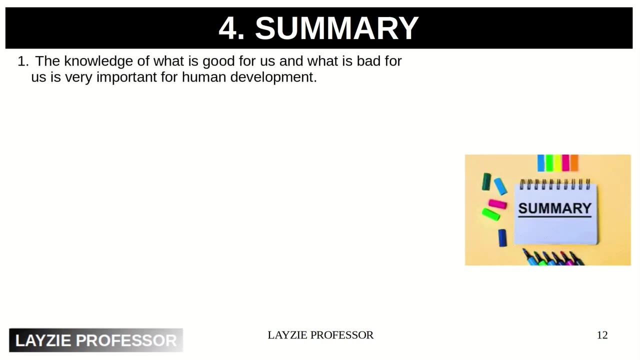 expressing and preserving this knowledge. Mathematical expression of knowledge is done in the form of theories, equations, graphs, etc. These are the bedrock of all the technological advancements we have made. The knowledge of what is good for us as human beings and what is bad for us is very important. 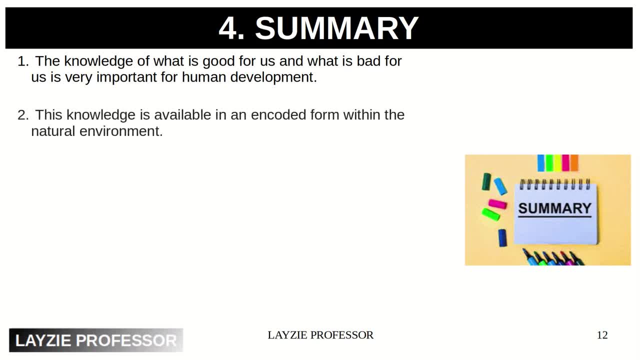 for our development and survival. This knowledge is available, but in an encoded form, within the natural environment we find ourselves in. Mathematics is a universal language which helps us to decode this knowledge. It helps us to express the relationships between the different elements that we find within nature. 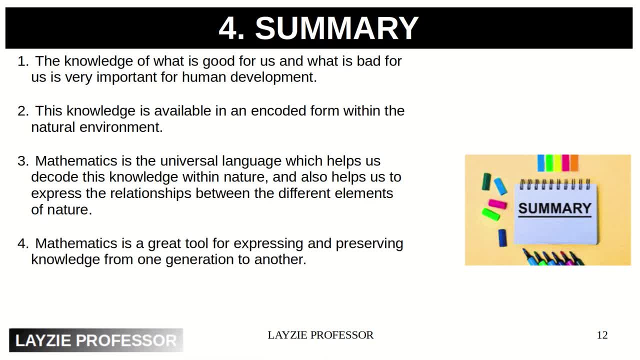 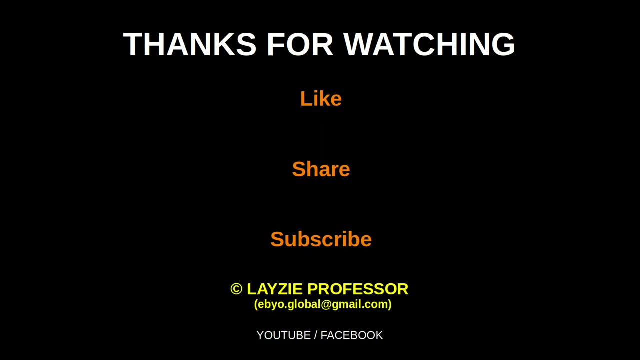 Mathematics is a great tool for expressing and preserving knowledge from one generation to another generation. This knowledge that needs to be preserved for human survival usually is expressed as theories, equations, graphs, etc. At this point, I would like to thank you For making time to watch my presentation. 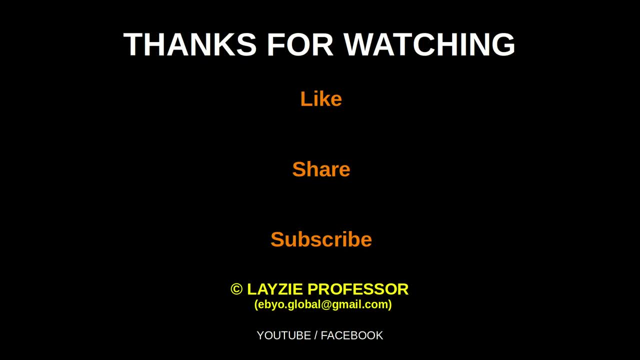 Please like, share and subscribe to my channel, Thank you.